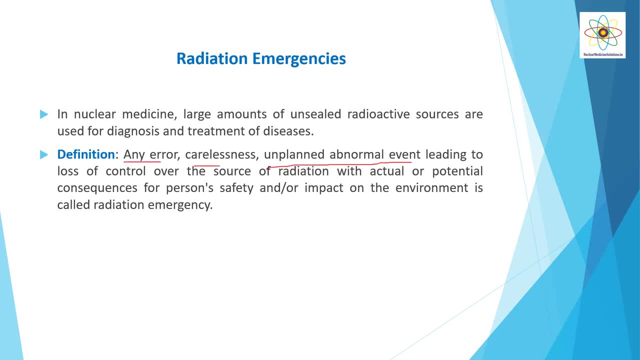 In this video we will learn about handling of radiation emergencies which we may face during our day-to-day working. This will include actions as first responder, actions as a subject expert- that is, by RSO Incineration Safety Office, and actions as a subject expert- that is by RSO Incineration Safety Office. and actions as a first responder. 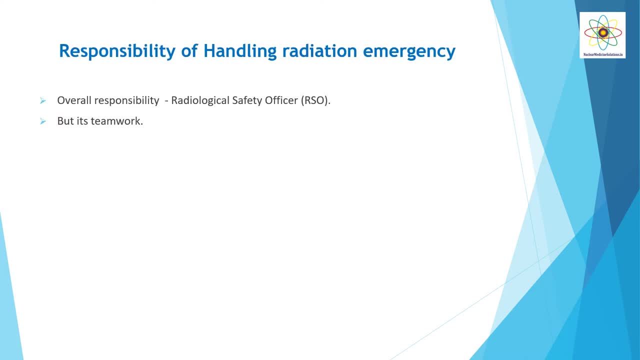 In this video we will learn about handling of radiation emergencies which we may face during our day-to-day working. This will include actions as first responder, actions as a subject expert, that is, by RSO Incineration Safety Office, and actions as a first responder. 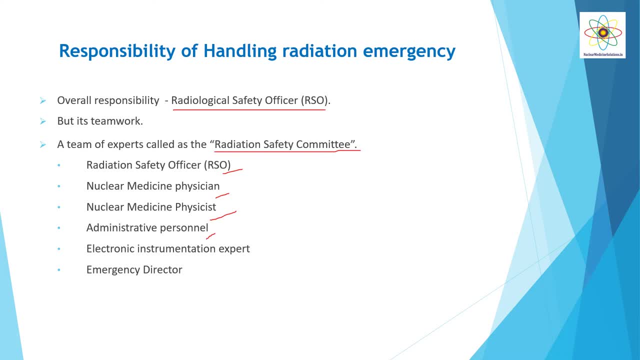 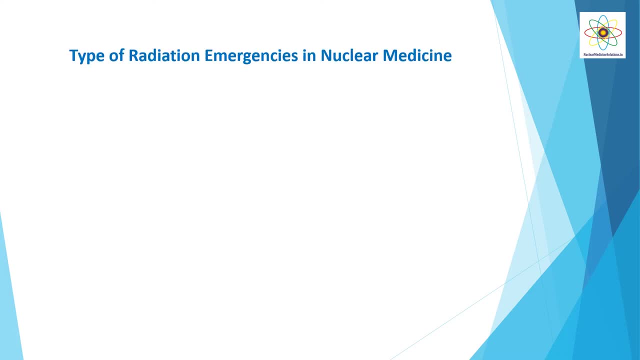 In this video we will learn about handling of radiation emergencies which we may face during our day-to-day working. This will include actions as first responder, actions as a subject expert- that is, by RSO Incineration Safety Office, and actions as a subject expert- that is by RSO Incineration Safety Office. and actions as a first responder. 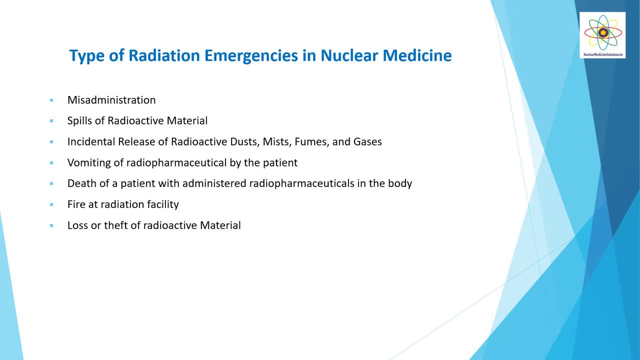 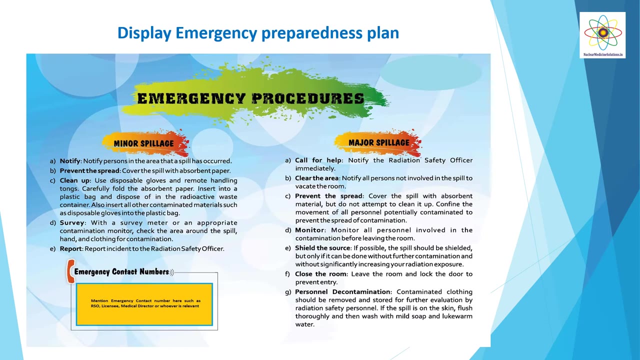 In this video we will learn about handling of radiation emergencies which we may face during our day-to-day working. This will include actions as first responder, actions as a subject expert- that is, by RSO Incineration Safety Office, and actions as a subject expert- that is by RSO Incineration Safety Office. and actions as a first responder. 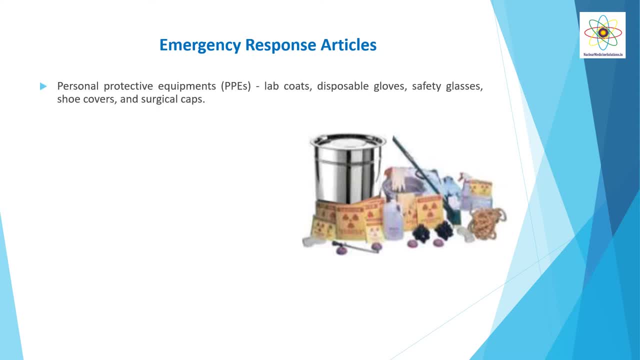 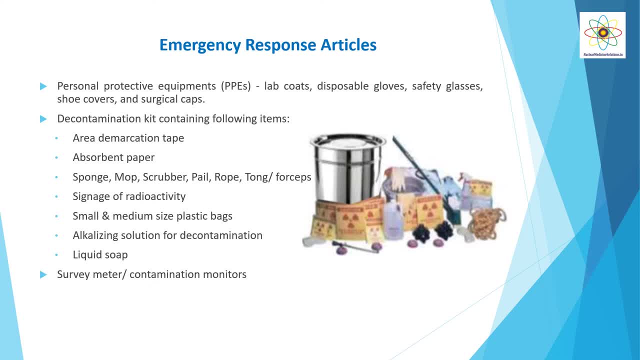 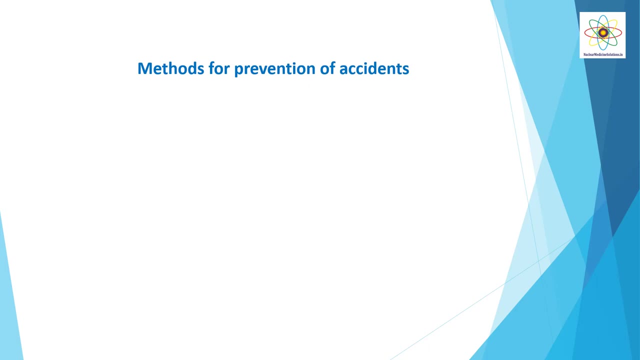 for decontamination liquid soap. There are some equipments also required, like survey meter or contamination monitor and emergency preparedness plan. As RSO, our first attempt is to prevent such incidents so that no one is at risk. There are methods to prevent radiation emergencies. 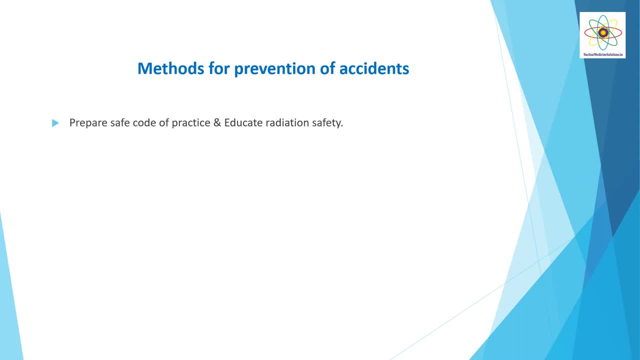 which are as follows: Prepare safe code of practice and educate radiation safety. Identify emergency situations and plan to avoid such situations. Any accidents happenings in the department should be attended to immediately and reported. Educate number of trained staff should be available to carry out emergency plan. 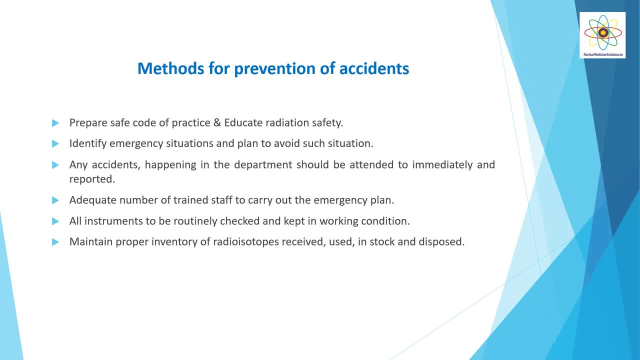 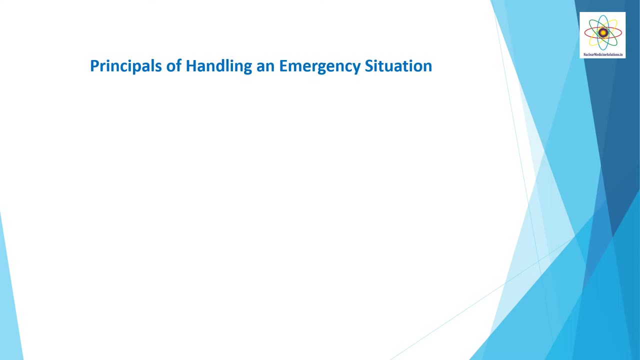 All instruments to be routinely checked and kept in working condition And, last but not the least, maintain a proper inventory of radioisotopes received, used and stocked and disposed. Now, despite all such preventive methods, some incidents are bound to happen. 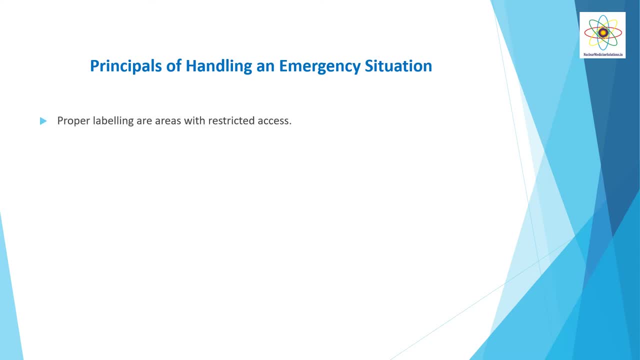 Then what are the principles for handling such situations? First, the proper leveling of areas with restricted access. Emergency contact information to be pasted in the area of use. Readily available decontamination kit and personal protective equipments for handling spills. Regular radiation safety training. 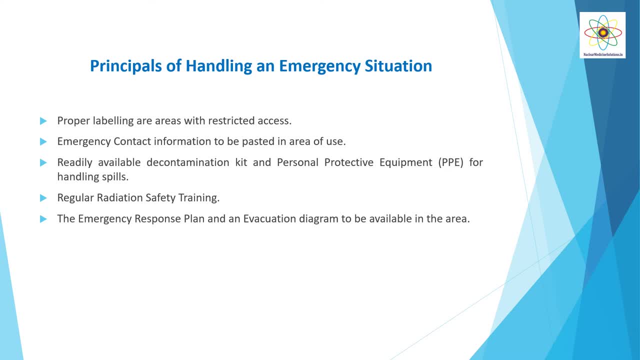 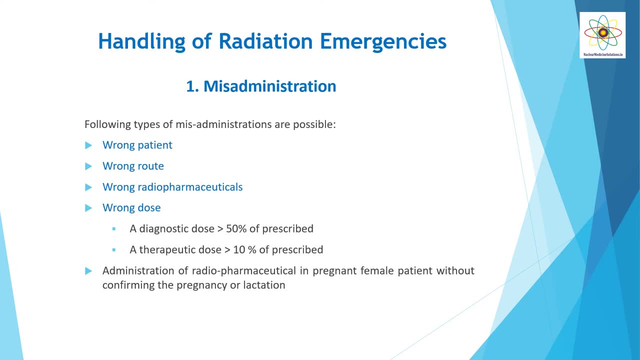 And the emergency preparedness plan and evacuation diagram to be available in the area. Let's discuss the handling of radiation emergencies First. let's start with misadministration. Following types of misadministration are possible. First, administration of radiopharmaceuticals. 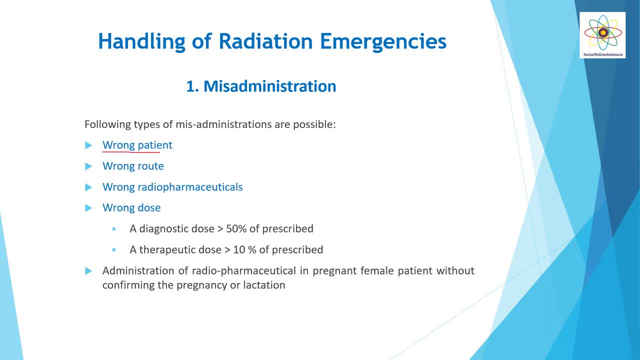 to a wrong patient. Administration through a wrong route, that is, oral, intravenous or muscular injection. Administration of wrong radiopharmaceuticals. Administration of wrong dose, that is, a diagnostic dose is more than 50% prescribed and a therapeutic dose more than 10%. 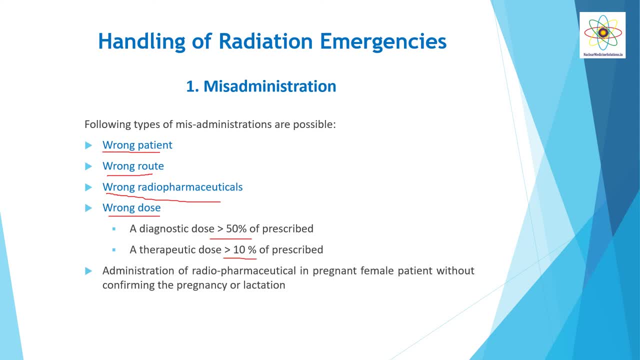 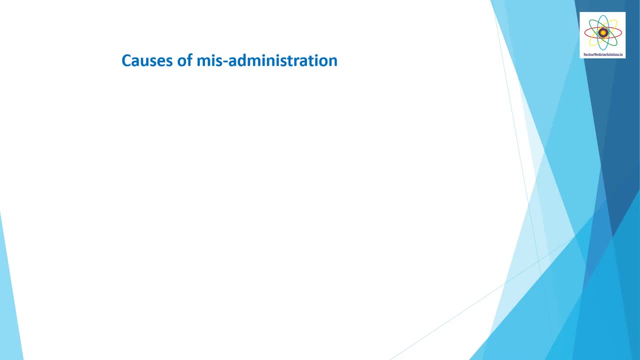 Finally, it is possible to perform 10 percent of prescribed and administration of radiopharmaceutical in pregnant female patient without confirming the pregnancy or lactation. let's see what are the causes of misadministration. first, there might be a communication problem or a gap, busy environment or distractions bypassing local rules or code of practice. 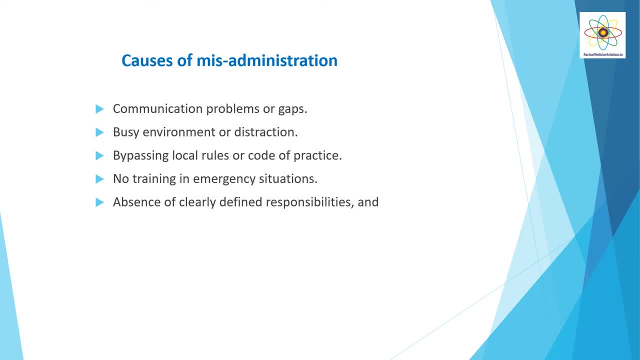 no training in emergency situations, absence of clearly defined responsibilities and absence of efficient quality assurance program. so how can we prevent such misadministrations? the chances of misadministration can be reduced by adopting standard operating procedures of following minimum points as mentioned below: tagging and segregating the vials and syringes with proper labeling. writing the amount of activity. name of: 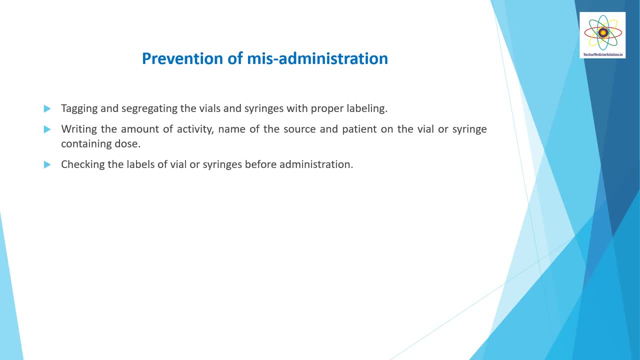 source and patient on the vial or syringe containing doses. checking the levels of vial or syringes before administration. measuring the activity and identifying the source before administration. proper identification of name number and the case of patient with case file and ensuring that female patient is not pregnant. now suppose, despite having all these, 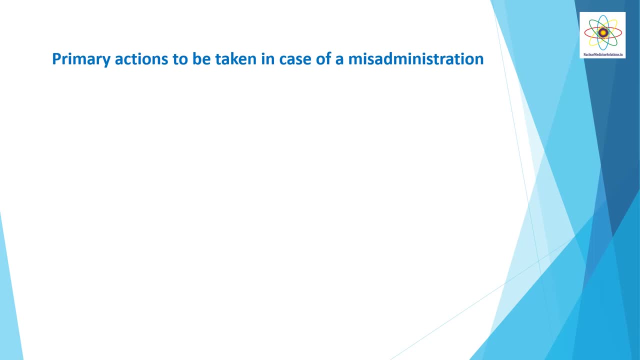 primitive methods, some misadministration occurs. so what are the actions we are supposed to take immediately? take actions to minimize any misadministrations and prevent misadministrations, and prevent misadministrations in general, as we're using 찔러에서 벽 걸으면 긴 방역에 따라 진지한 고려의 구조가. 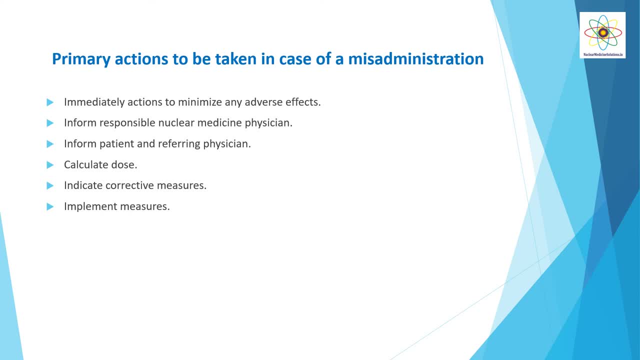 질산 정보를 제한하시는 것이다. we have a separate class on how to calculate those in patients. you can subscribe to the channel and press the bell icon to know the notification and future classes. once initial management is done, inform head of department, licensee and regulatory authority through incident retention and. 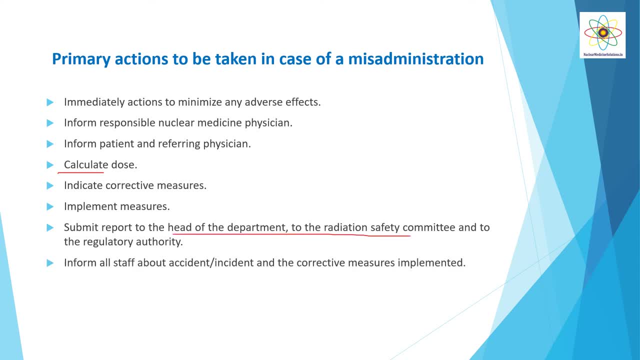 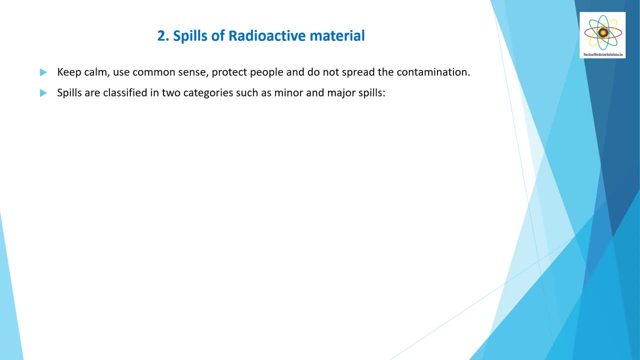 ruptures are always in place by the department, so we need to get regardless of that and we need to reporting. In forthcoming slides, I'll let you know the procedure for incident reporting and the timeline. Now let's discuss spills of radioactive material. All efforts are to be made to avoid 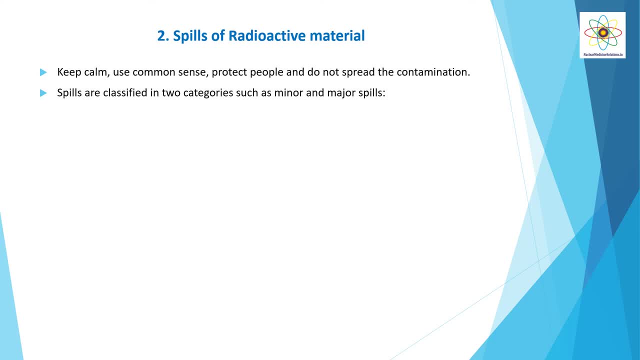 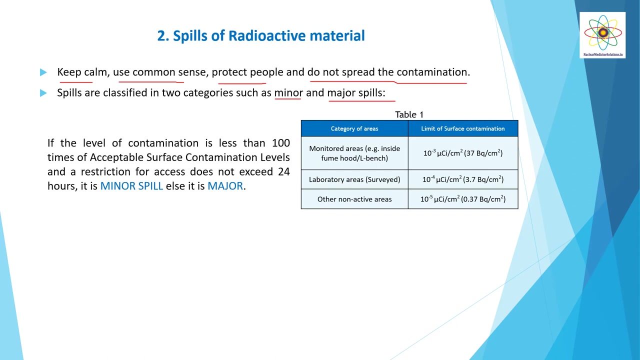 spill of radioactive material. However, in the event of accidental spillage, keep calm, use common sense, protect people and do not spread the contaminations. Spill is classified in two categories: One is minor and the other is major If the level. 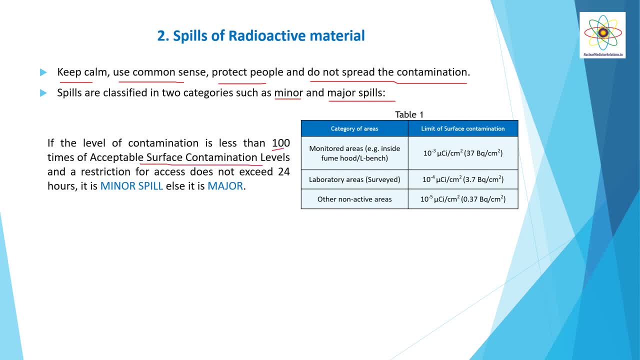 is contamination is less than 100 times of acceptable surface contamination level and a restriction for access does not exceed 24 hours. it is minor spill, otherwise it is a major. The limit of surface contamination of various areas, like level of contamination inside fume hood or L bench, inside laboratory area or a non-active area, is shown in the. 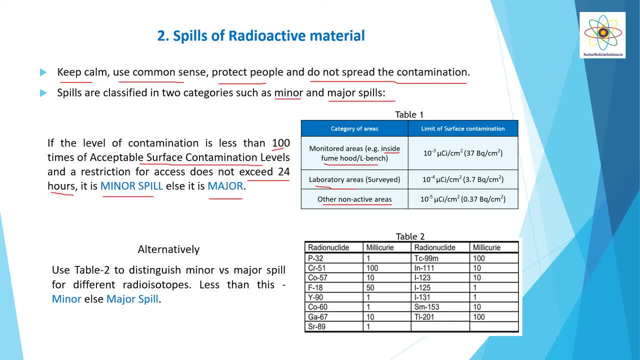 table. Alternatively, table 2 can be used to distinguish minor vs major spill for different isotopes. If less than this activity it is a minor spill, else it is a major spill. Like a technetium-99m has fallen on less than 100 mq, then it will be a minor spill, and if it is more than this 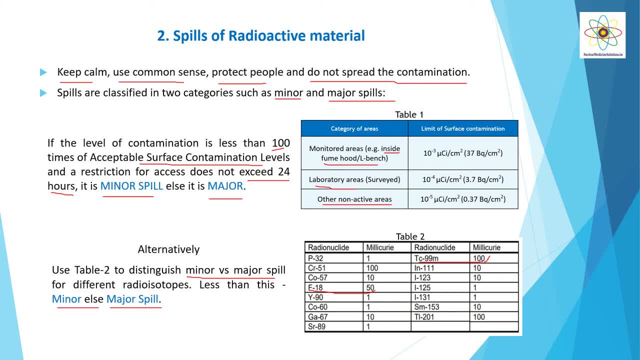 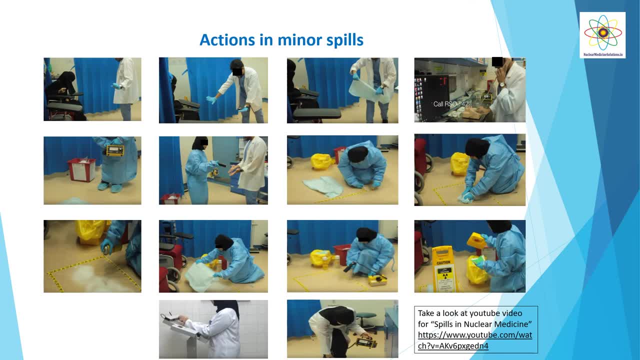 it will be called as a major spill For F18, the limit is 50 mq. Likewise it is given for other isotopes which are used in nucleoviricin. Handling technique of both minor and major spills is different. The procedure of handling should be known to the person who see it first. 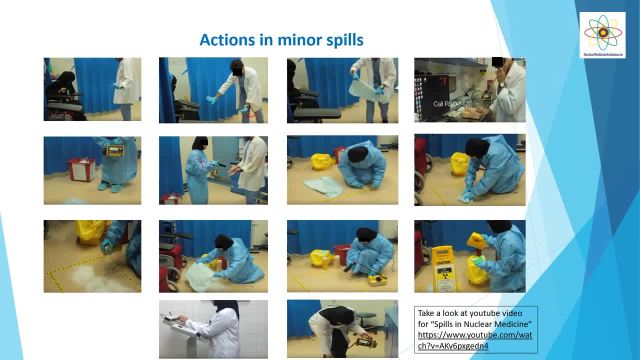 that is, by the first responder and by the subject expert, that is, by RSO. Let's see how to manage spills of radioactive material. There is a YouTube video made by Ms Fatima on spills in nuclear medicine. You can go through by searching it. The link is: 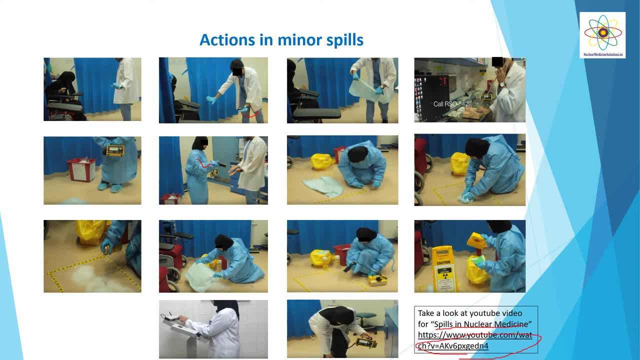 shown in the slide. Few images are picked to showcase management in pictorial version for easy understanding. I express my sincere thanks to Ms Fatima for this video. In the picture, the authorized person going to inject RadiotHD system of the patient and suddenly syringe fell and radioactivity spilt immediately. 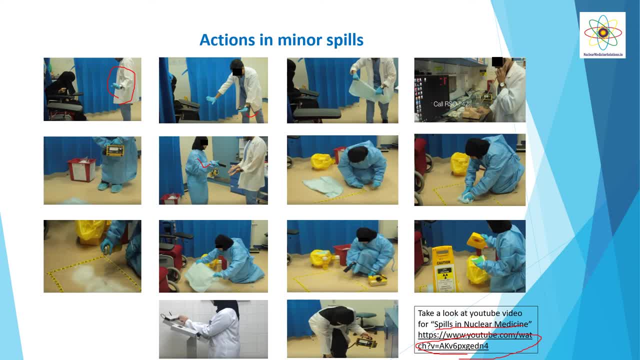 he stopped the movement around to prevent a spread Contained Ready Activity by keeping Abvers punishment sheet onto eight and inform RSO on arrival. RSO Wish you cover disposable gown and gloves. She should also wear mask and cap. She won't double gloves for extra. 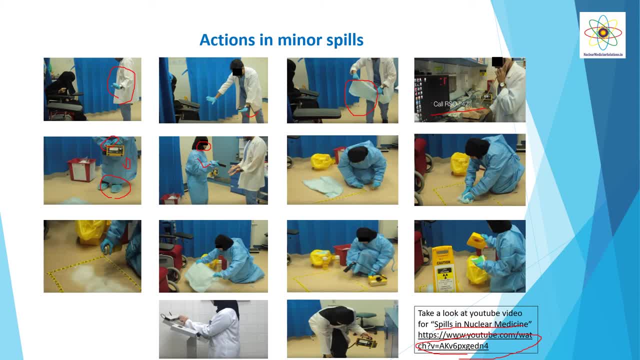 precautions. She picks up the survey mater and ask for the contamination kicked. she surveys the area. She pick up the survey and ask for the contamination kit. She surveys the area and post prax talent around Now while handling a spill. she marks the area with demarcation tape and picks up the spread absorbing sheet. 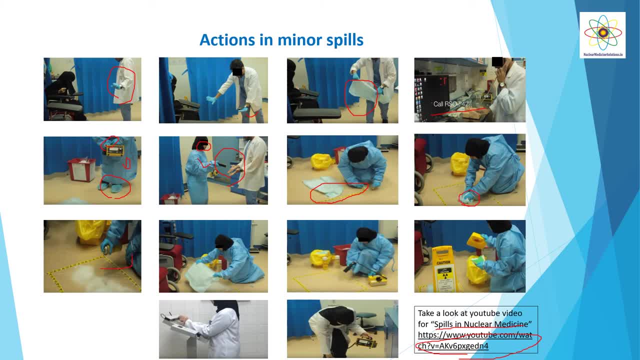 While picking up, be cautious about not spreading the contamination. She sprays contamination solution and cleans the area. While cleaning wipe the area from outer to inner. All contaminated material is kept in a plastic bag and labeled properly as radioactive waste. After cleaning, she surveys the area again and if any trace is found, she needs to repeat the procedure of cleaning again. 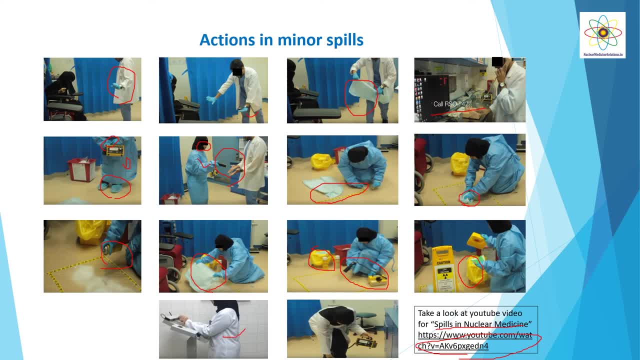 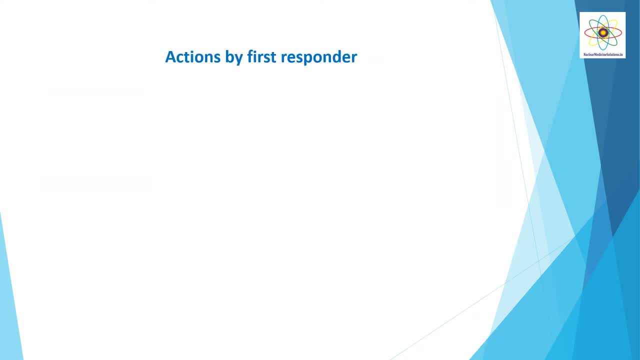 After that, she carefully removes her disposable clothings and surveys herself thoroughly. We will see these steps as bullet points in next slides. So lets see actions by first responder. Confine the spill immediately by dropping paper, towel or other absorbent material on it. 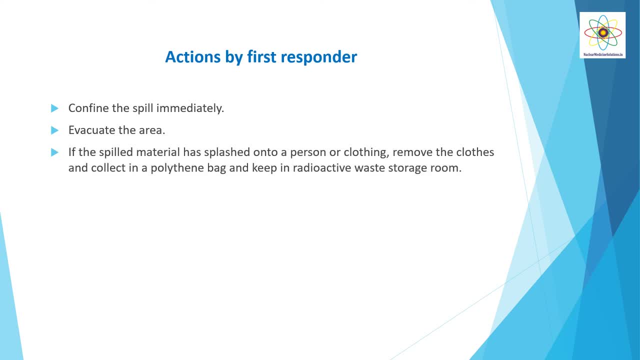 Evacuate the area immediately So that persons will not walk over the spill and spread the contamination. If the spilled material has splashed onto a person or clothing, Remove the cloths and collect it in a polythene bag and keep it in radioactive waste storage room. 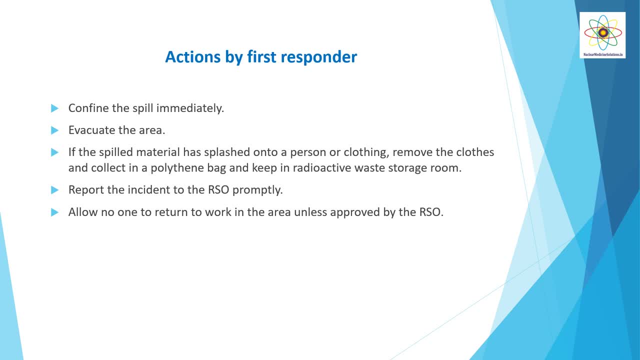 Report the incident to the RSO promptly. Allow no one to return to work unless area is approved by the RSO. Now cooperate and follow instructions of RSO. Now the actions by RSO in a minor spill: Call for decontamination kit. 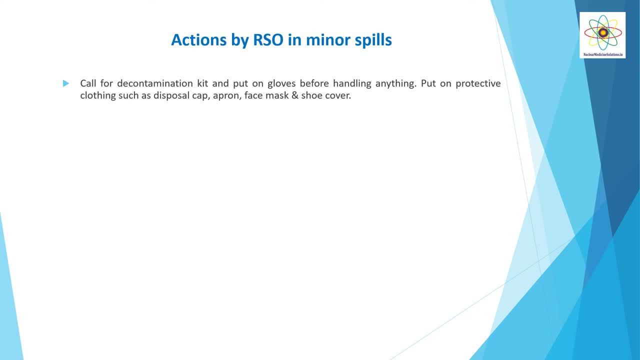 Put on gloves before handling anything. Put on protective clothing such as disposable cap, apron, face mask and shoe cover. Cordon off the spill area with demarcation tape. Wipe the area from outer to inner and fold contaminated paper with clean side out. 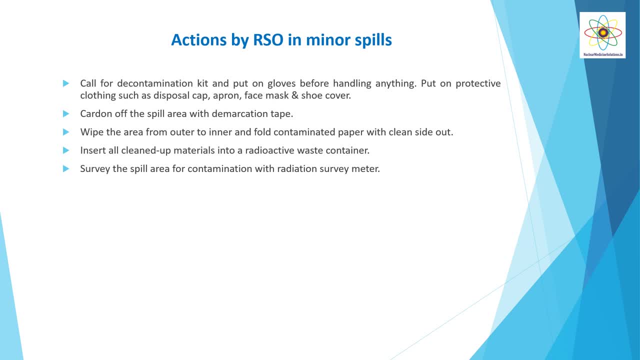 Insert all cleaned up material into radioactive waste container. Survey the spill area for contamination with radiation survey meter. If contamination persists, repeat the cleaning procedure again. Take wipe test to check any removable contamination. Once all done, remove protective clothing and store it in a radioactive waste label container. 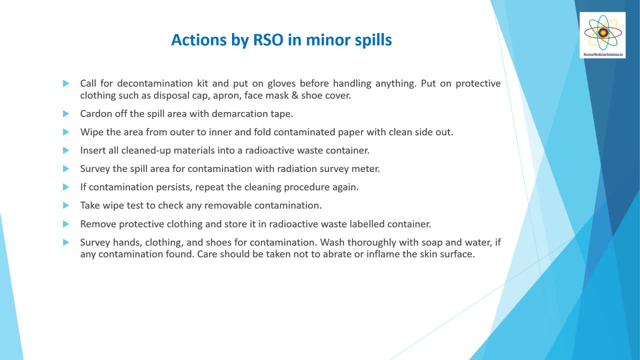 Survey hands, clothing and shoes for contamination. Wash thoroughly with soap and water. if any contamination found, Care should be taken not to abrade or inflate the skin surface. if there is any contamination found, Document entire proceedings Determine cause and appropriate corrective actions needed to avoid. 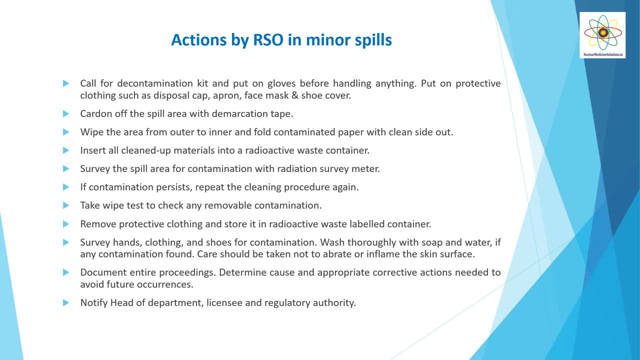 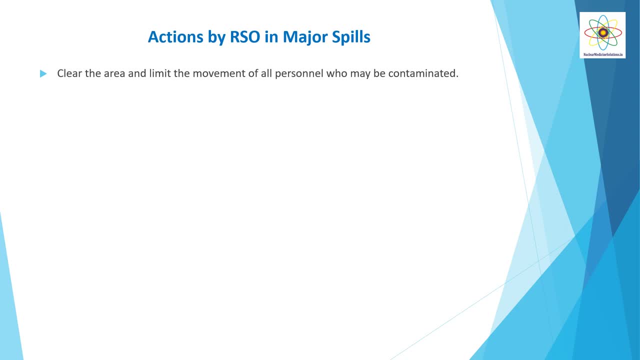 Future occurrences and then notify head of department, licensee and regulatory authority. Now we will see actions by RSO in a major spill. Clear the area and limit the movement of all personnel who may be contaminated. Prevent the spread of contamination by covering the spill with absorbent paper, but do not attempt to clean it up. 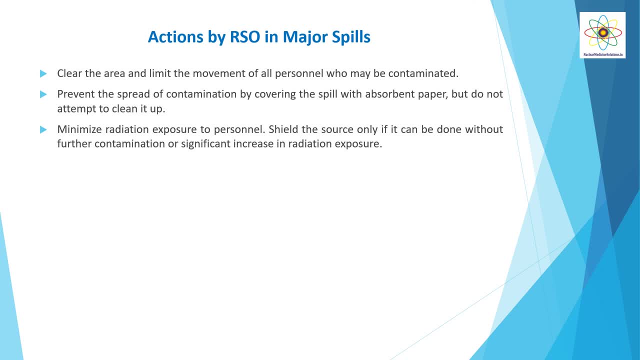 Minimize radiation exposure to personnel. Shield the source only if it can be done without further contamination or contamination Or significant increase in radiation exposure. Close the room and lock or otherwise secure the area to prevent entry. Post the room with a sign to warn anyone trying to enter that a spill of radioactive material has occurred. 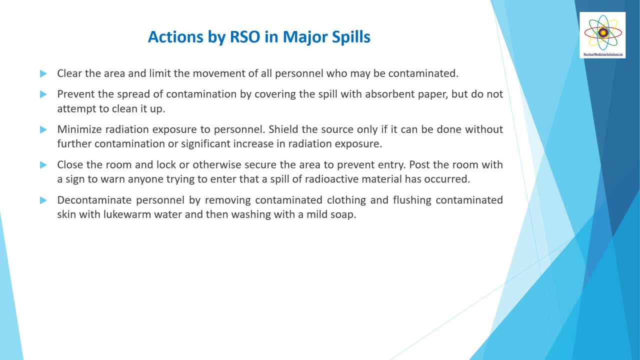 Decontaminate personnel by removing contaminated clothing and flushing contaminated skin with lukewarm water and then washing with a mild soap. Consider need for bioassay if radioactive material is suspected to have been contaminated. Determine cause and appropriate corrective actions needed to avoid. 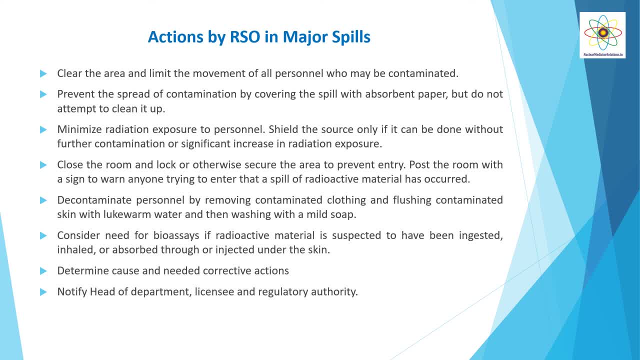 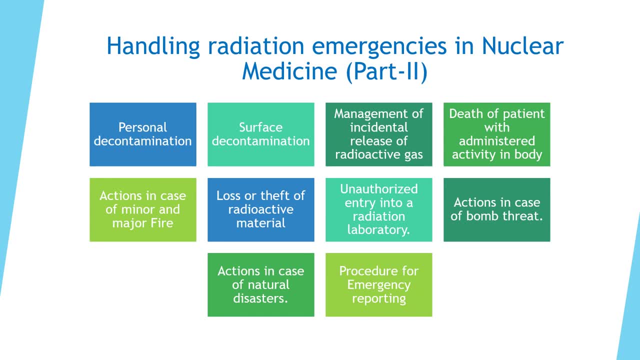 Notify head of department, licensee and regulatory authority. Determine cause and appropriate corrective actions needed to avoid. Notify head of department, licensee and regulatory authority. We will stop this video here And in second part of this video we will discuss personal decontamination, which will include external as well as internal decontamination. 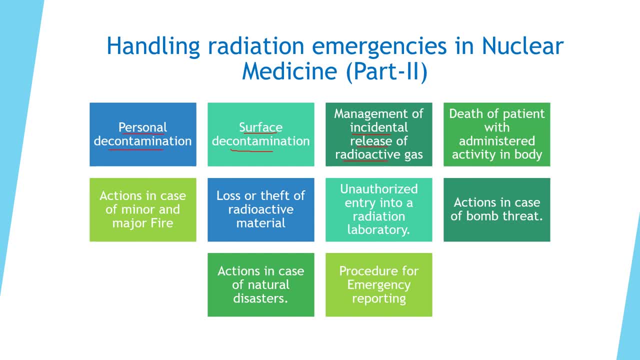 We will see how a surface decontamination can be done. We will see management of incidental release of radioactive fume gas or dust Actions as RSO in case of death of patient with administered activity with limits of disposal. We will also discuss actions in case of minor and major fire.